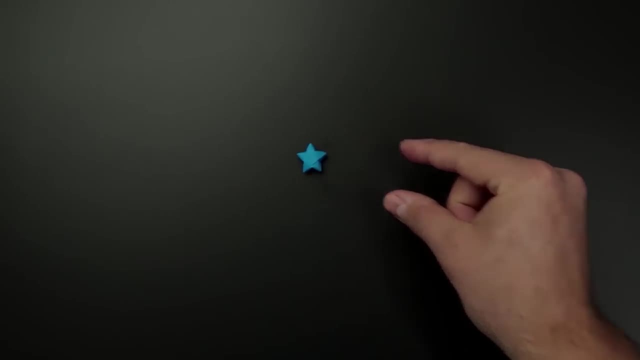 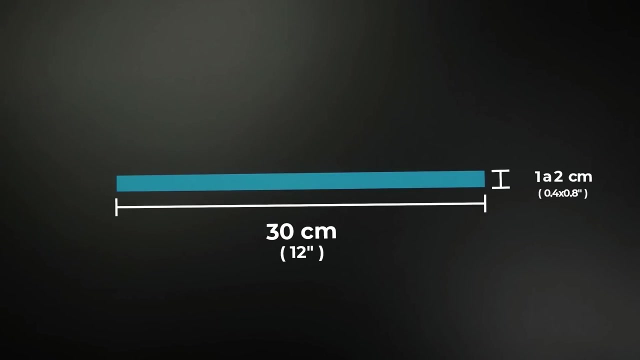 The size of this rectangle can vary, but for a better result I recommend to use at least 30cm wide and 1 to 2cm high. But, as I said, the size can vary. you can use any piece of paper you have as long it. 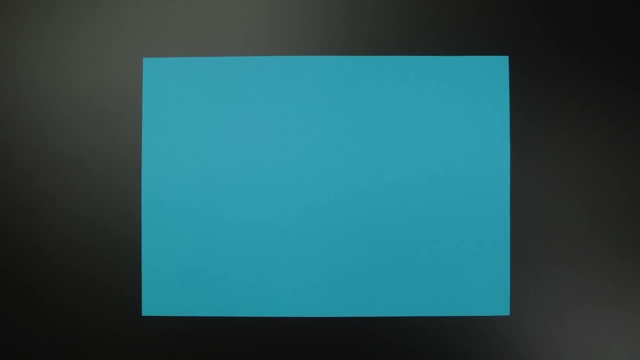 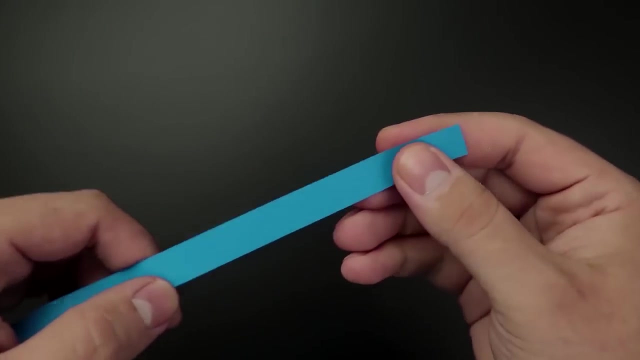 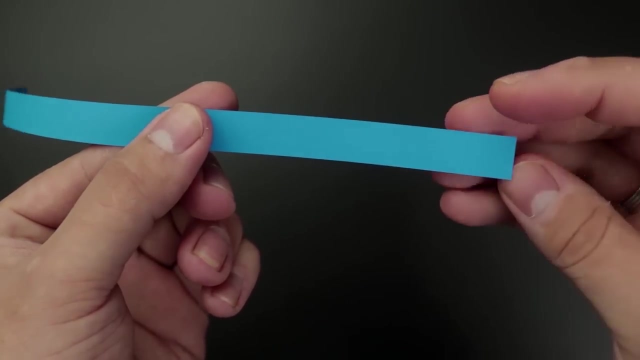 is a rectangle. To make it even easier, you can start with a whole sheet of paper and divide into 16.. Having this rectangle, our next step is to tie a knot on the right side. You just need to bring the right side up, making a lace or a loop. 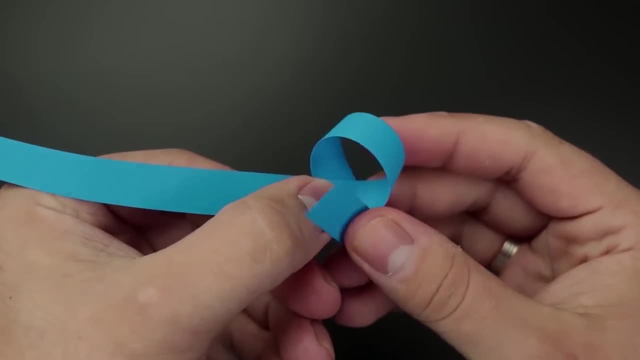 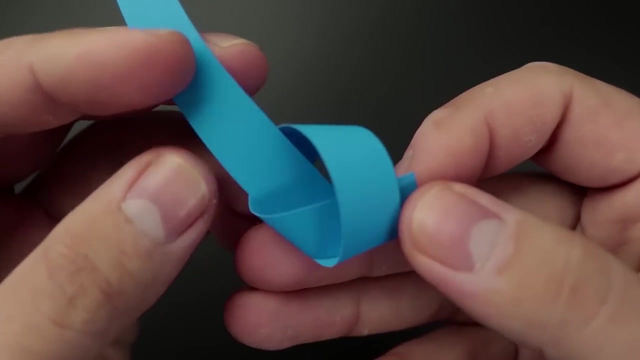 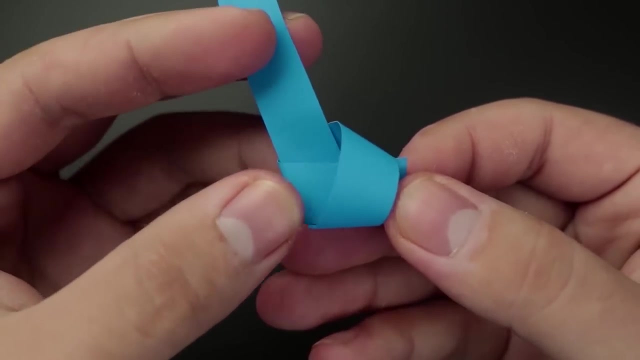 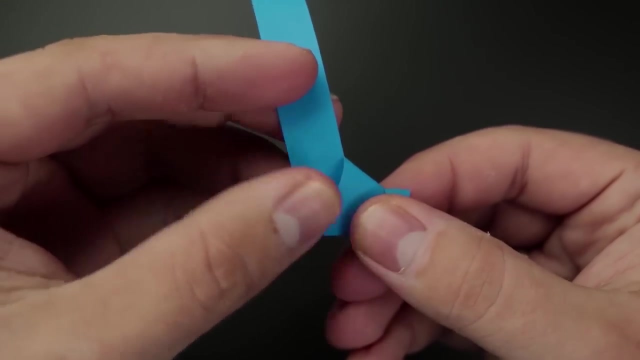 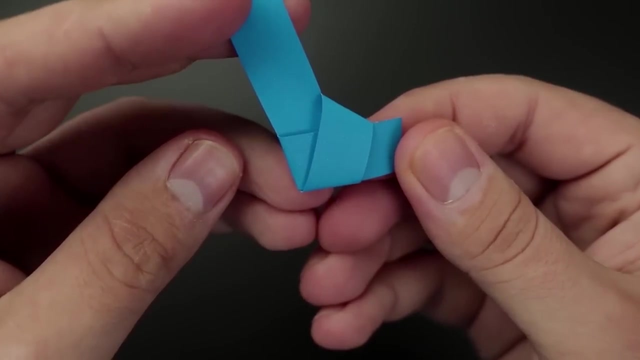 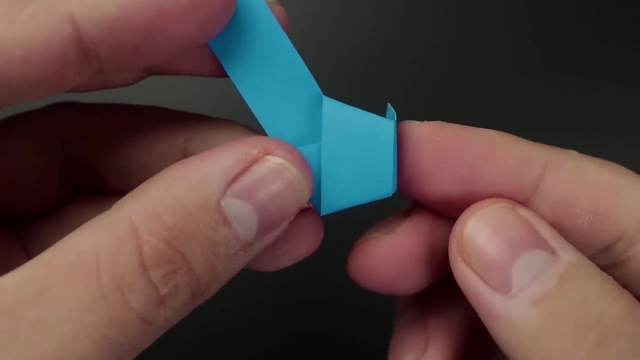 Now going through the middle And pull it very carefully, creating the knot. When it closes, we'll have something like a pentagon. You'll have a little bit of paper left over on the right. Let's fold it back, Creating one of the pentagon's edges. 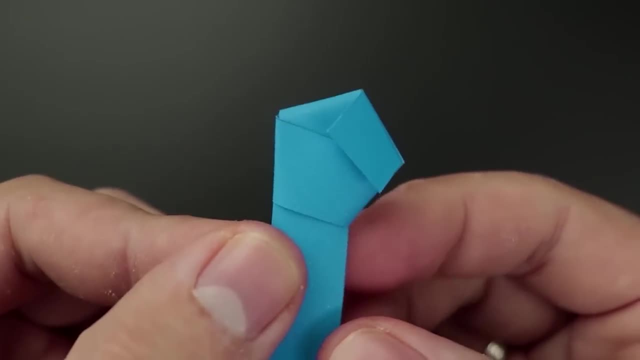 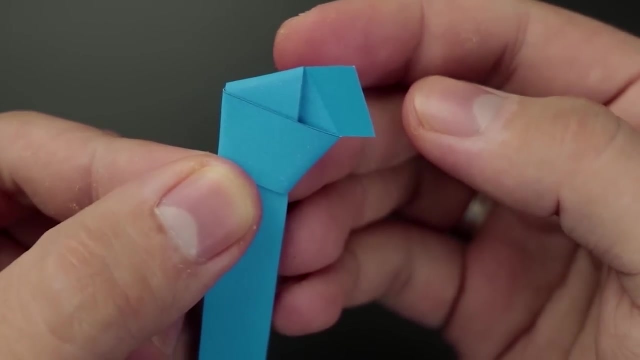 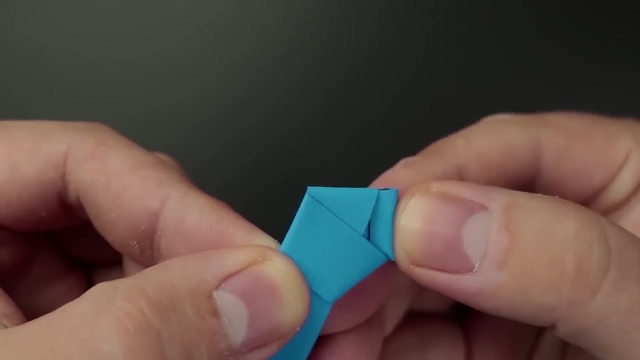 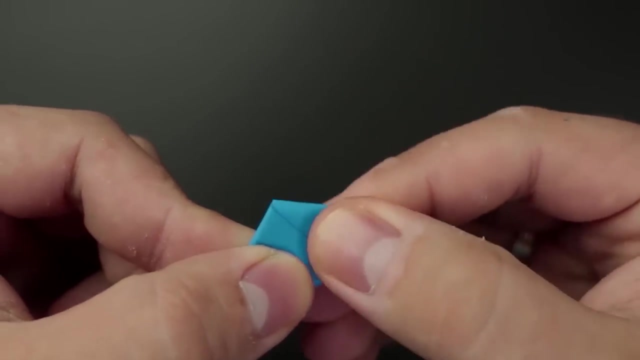 Now turn it over, Unfold And put the difference under the middle layers, And there you have it, our pentagon. It's done. Thanks for watching. See you next time. Let's go back to the other side Now. pay close attention. 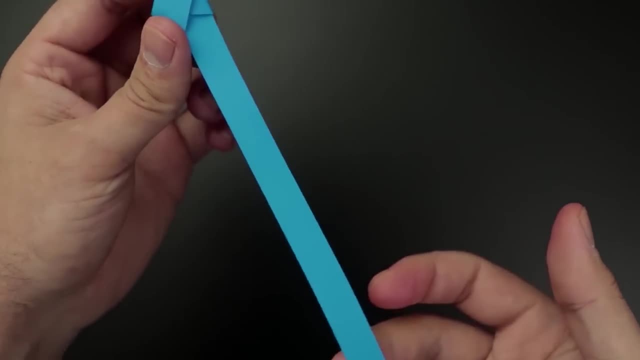 We need to fit this larger part Under the front layer. Don't forget to like and subscribe, And if you have any questions, let me know in the comments. I will be happy to answer them. See you next time. Bye, bye. 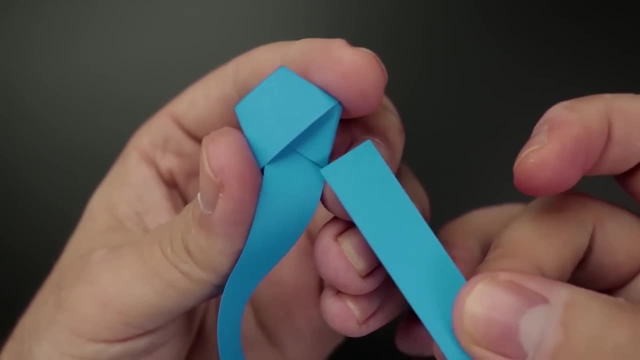 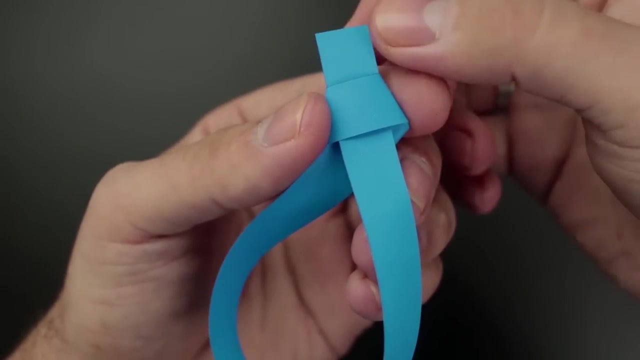 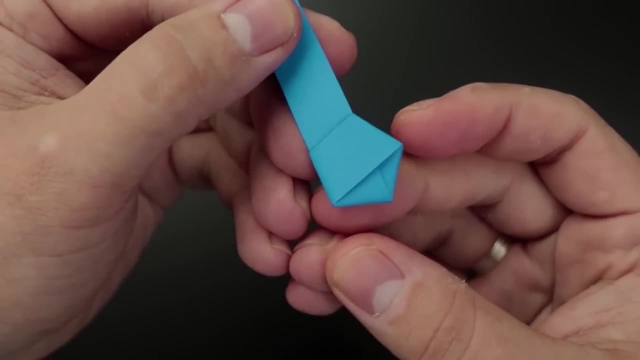 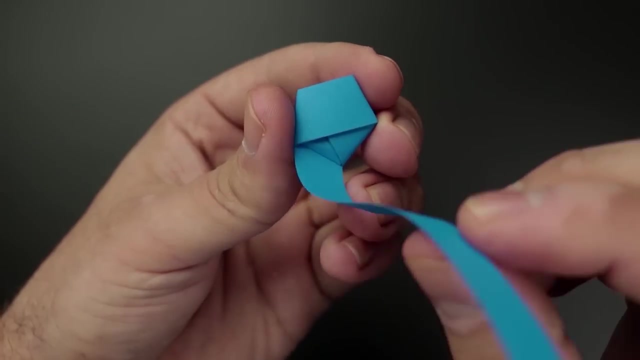 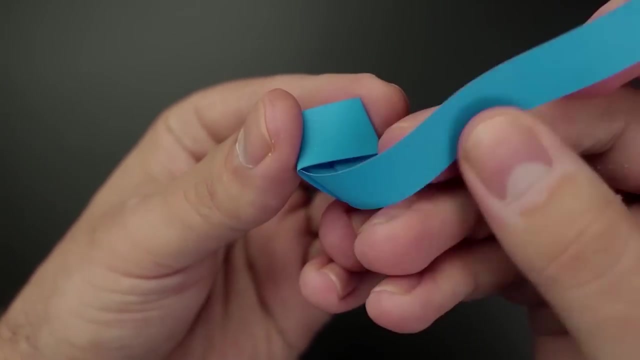 Bye, bye. the pentagon is closed. let's go to the other side. and now, to keep the pentagon shape, we are going to have to go over the top. throughout this process, there will be moments where the paper will go over and others under the layer on the 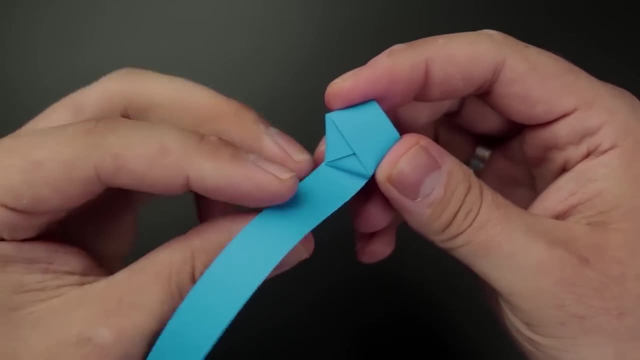 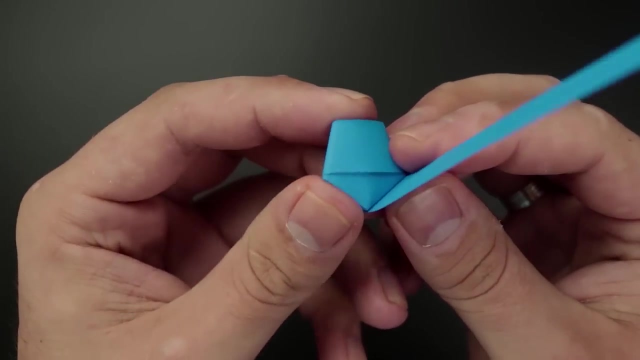 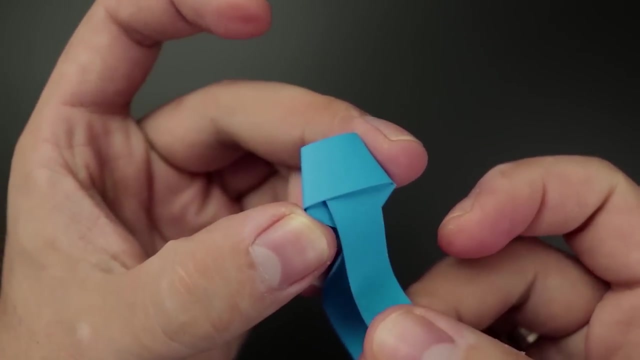 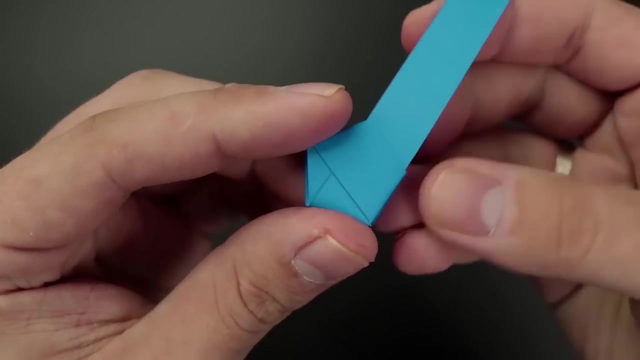 other side we'll do the same: just pass the paper over, but on the next we'll be able to put it under the layer. every time you do this, the paper will become more resistant. now that you know how to do it, just repeat the same logic until the end. 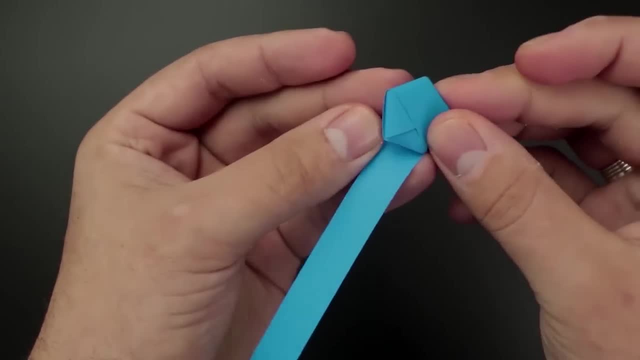 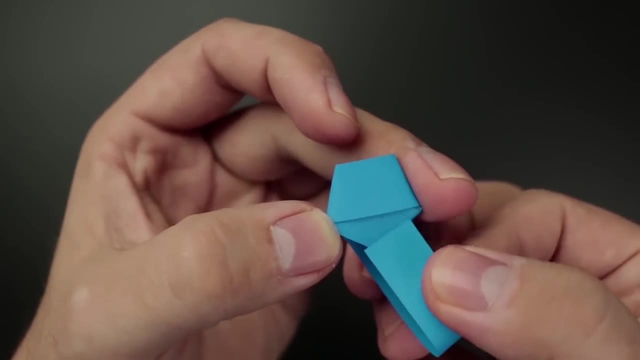 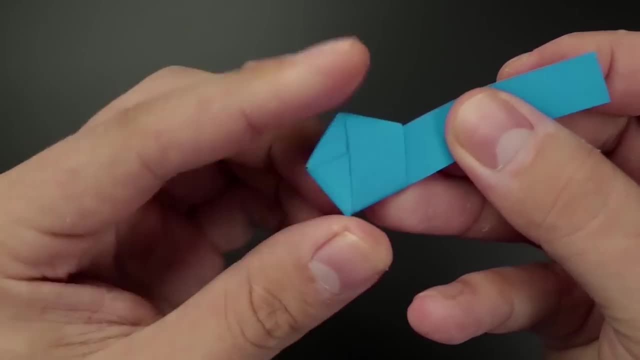 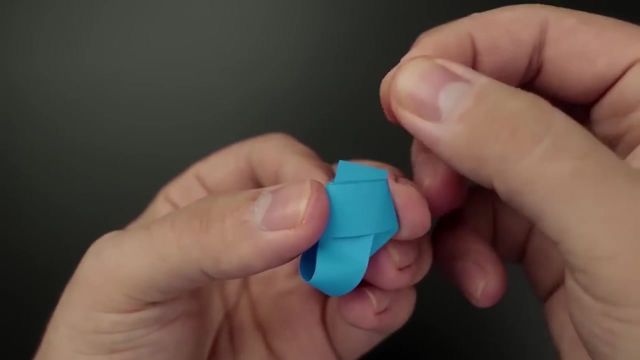 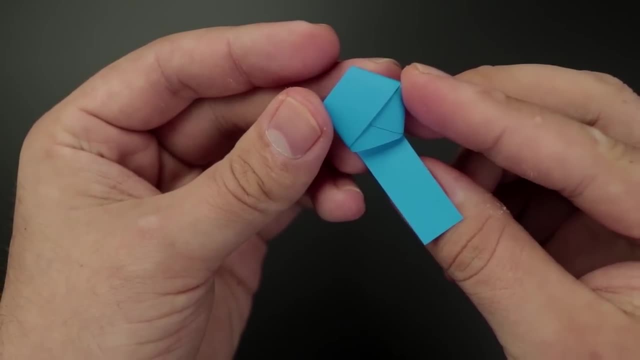 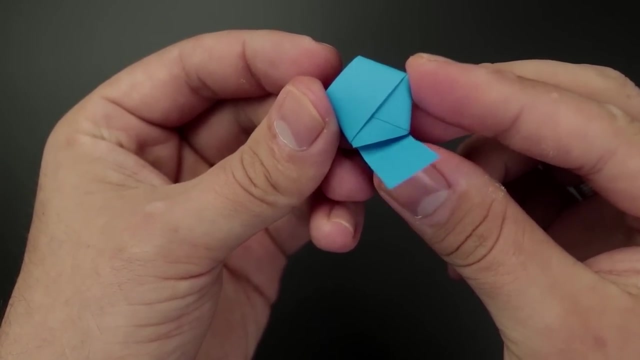 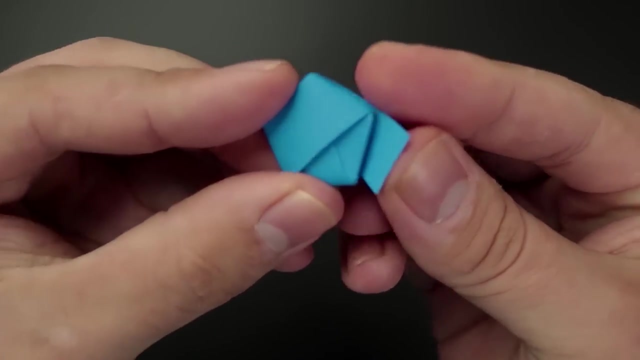 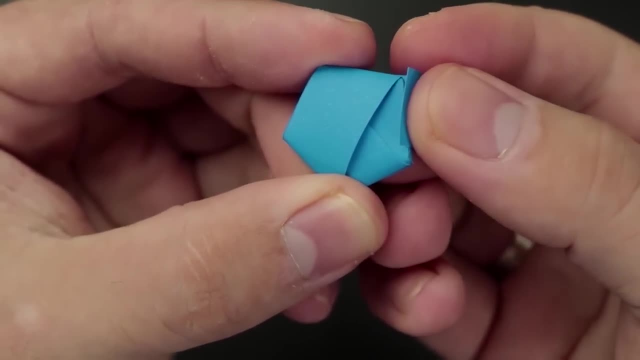 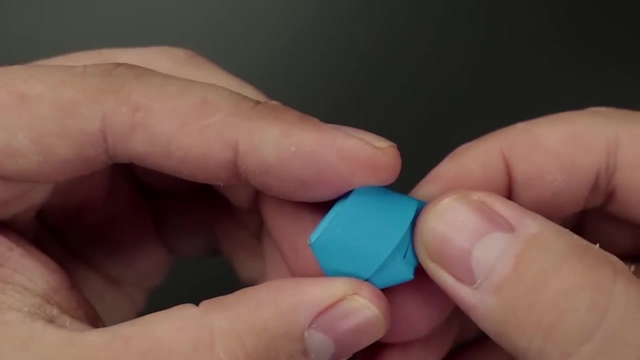 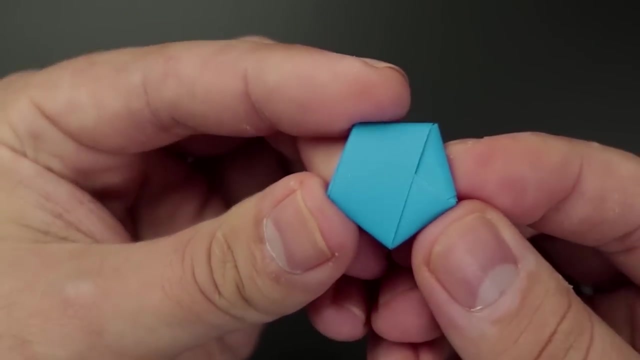 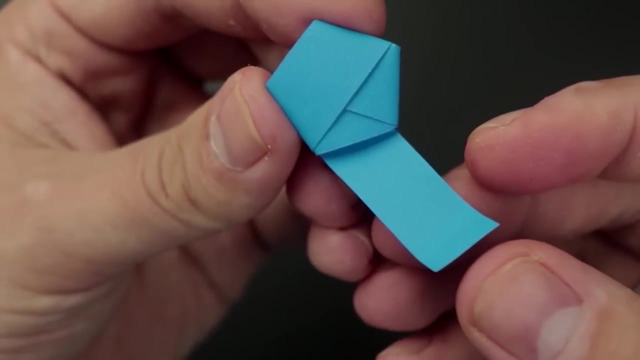 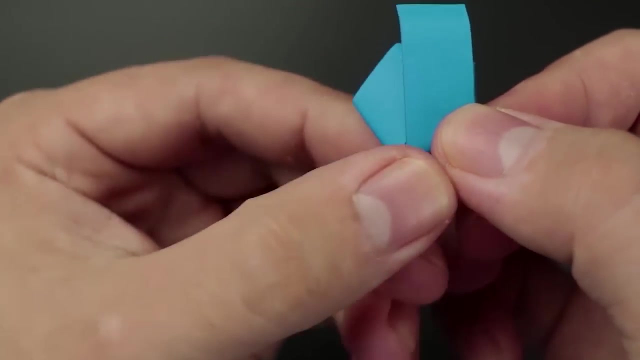 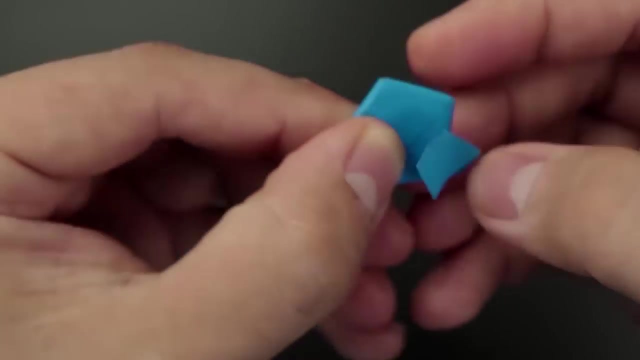 little bit of paper under the first layers, just like we did in the very beginning. you we have the Pentagon ready. the next option, the option I recommend, is to leave the paper a little more unfold, bring it over and then fold the difference to the middle, keeping inside the Pentagon. then just fit the paper.